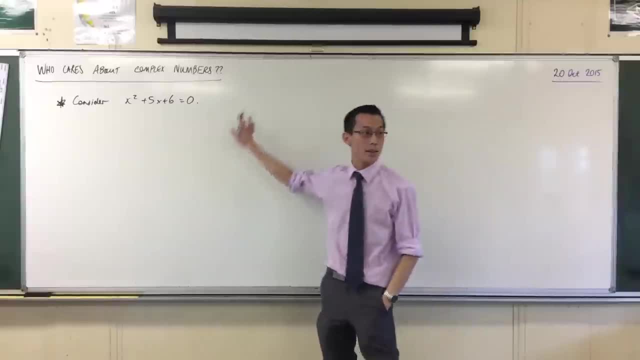 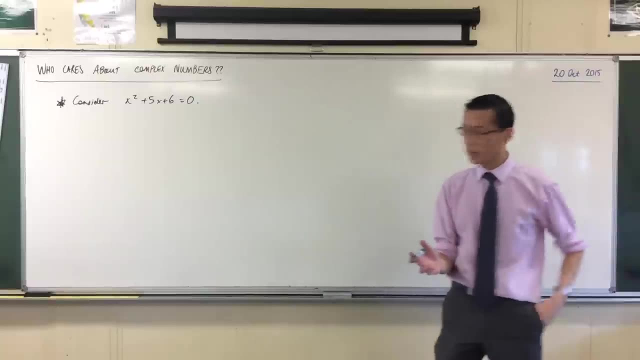 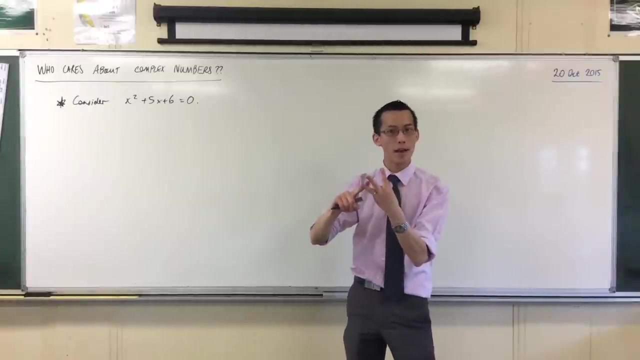 However, what I'd like to point out to you- and I'd like us all to rehearse it together- is, Normally you would solve this by factorising, because it's easy to factorise, right. But we go through factorising, then we go through completing the square and we use completing the square to arrive at the quadratic formula. okay, 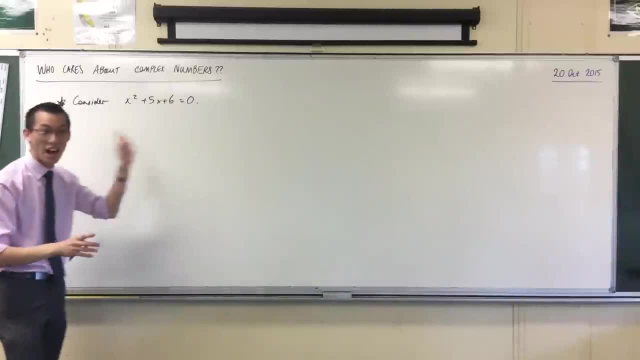 The quadratic formula is great because you know you can use it on anything, even when it's hard to factorise. So I want to take this and I want to just use that skill that we know about the quadratic formula. I just want to apply it to here. We know what the conclusion will be, but I just want to see what happens as we go through. okay, 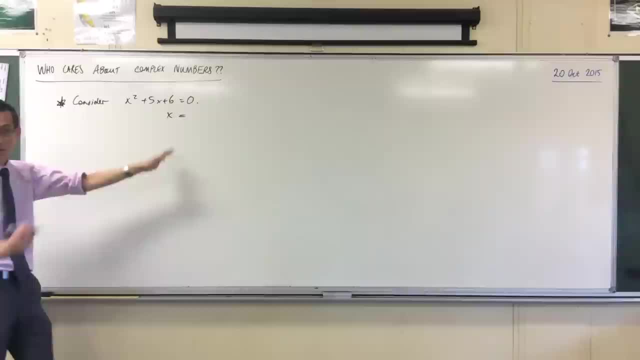 So human meaning. We know what the quadratic formula is. What number is it that I'm going to put in Minus 5.. Minus 5, which is b, plus or minus the square root of 5, 5 squared, which is 25.. 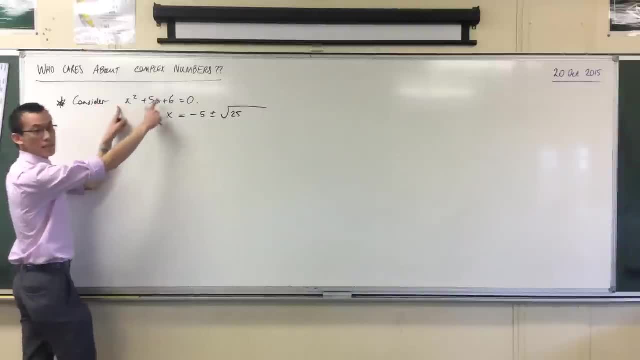 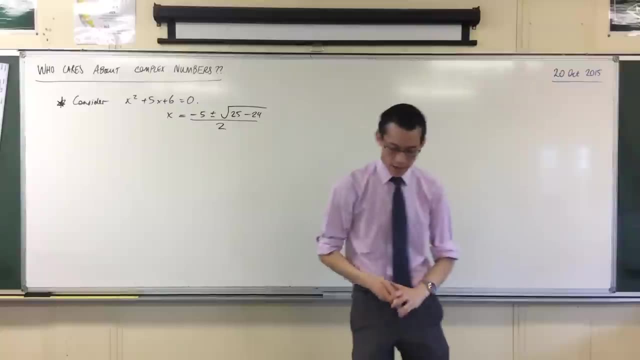 Minus 4ac, which is 4 x 1 x 6, which is 24.. All over, in this case, just 2.. Okay, are you happy with that? Now, what I want to point out to you before we go any further, is that, according to the quadratic formula, 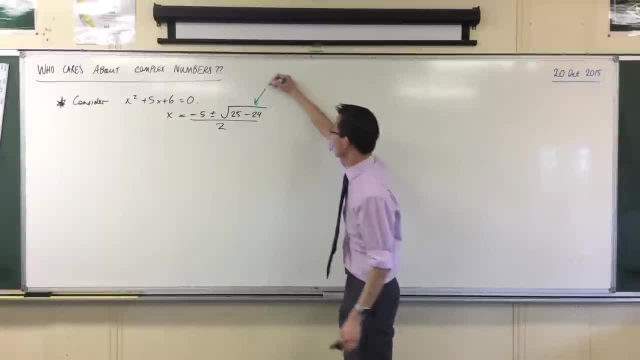 like quadratic formula has baked into it serves- right, It has serves like it's part of the formula. You have to say minus b, plus or minus the square root of. If you don't say the square root of, then you won't get the quadratic. 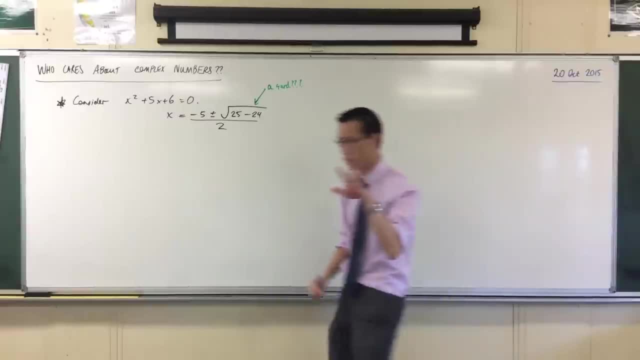 formula and you won't get the answers Now. just keep that in the back of your mind. Let's continue. 25 minus 24,, of course, is One One, And the square root of one is One One. 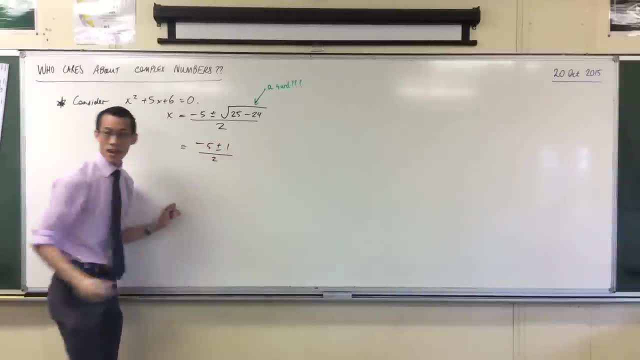 Okay, Yes, thank you. So I've got that in there, No problems. The reason why I don't need to worry about the absolute value is because I've got four cases anyway, right, And from here we're going to get well. 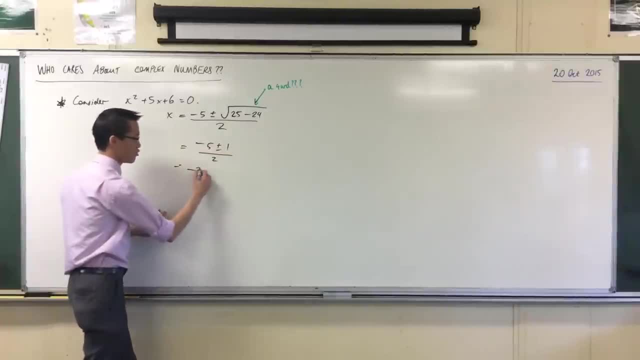 the negative case will be minus five, minus one which is minus six, So you get negative three. And the positive case will be minus five plus one which is negative four, So we get this solution. Now, this is weird. 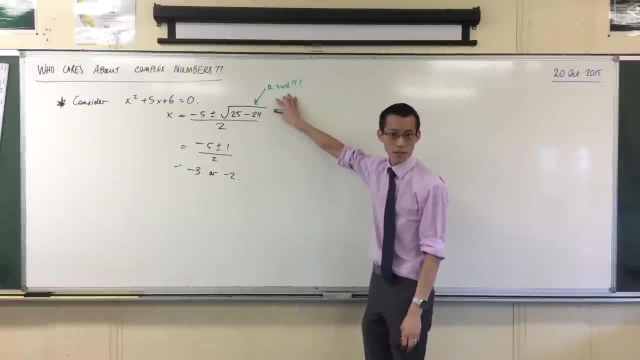 This is weird. The formula itself has a third in it, right? But then the third disappears Because you only get the positive result. It should be like plus minus, right? Sorry say that again. Like, so you know when you get third and one. 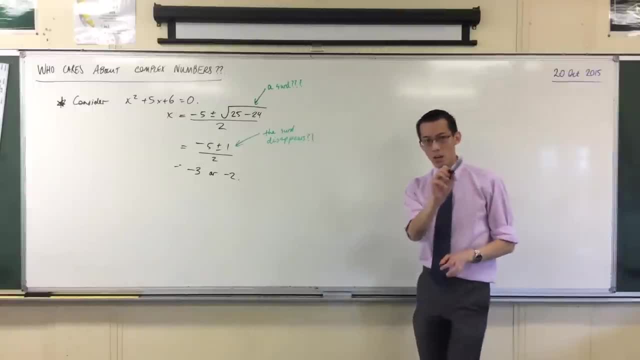 shouldn't you get like a plus minus one? Okay, Now, what you're talking about is getting a multiplicity of answers, like, how many answers do I get? But what I'm interested in is: what kind of answers am I getting? 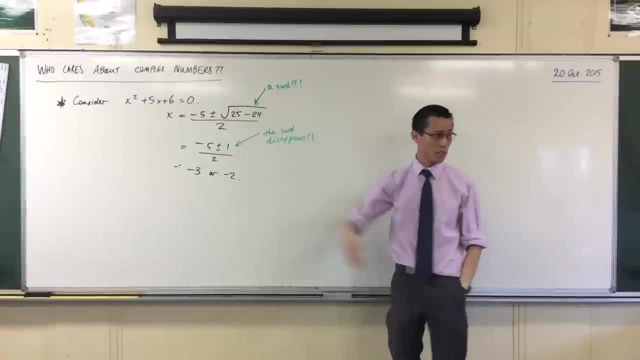 And the answer is: I seem to start off with a third. The formula tells me to expect a third, But then the third just kind of doesn't become a third, It just disappears. okay, Now, this is strange, right. 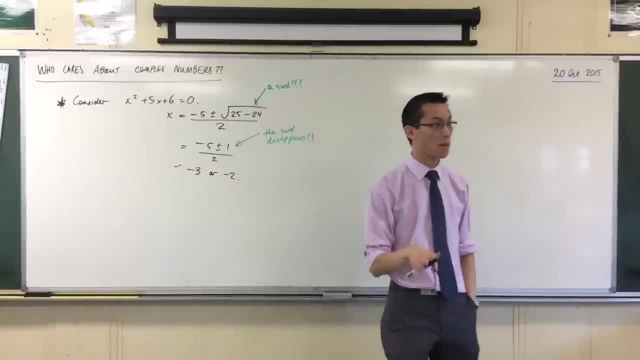 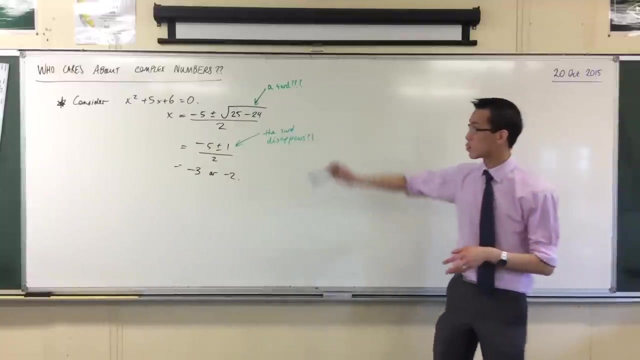 I have an answer that's completely rational, right? Whole numbers even in this case. But to get to these rational numbers, I have to appeal to irrational numbers, right? And they just seem to, you know, vanish away. Now, here's the important thing, and this is what starts. 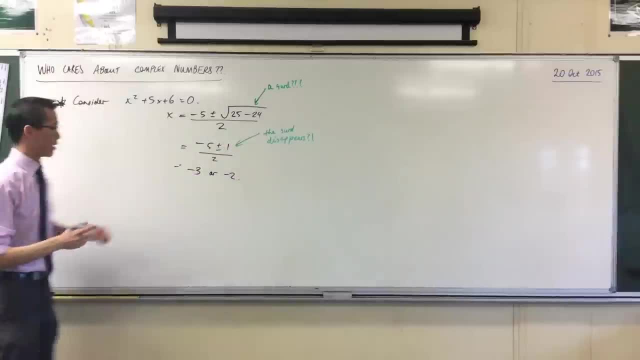 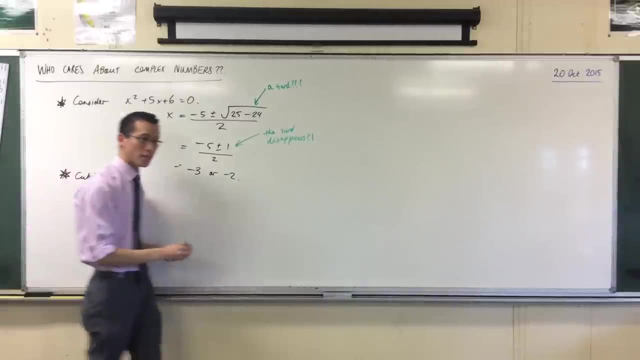 to answer this question for us. okay, This is a quadratic, This is a quadratic. I have alluded to the fact before that if you do not have a quadratic, but if you have a quadratic, you have a quadratic. If you have a cubic formula, right, if you have a cubic. 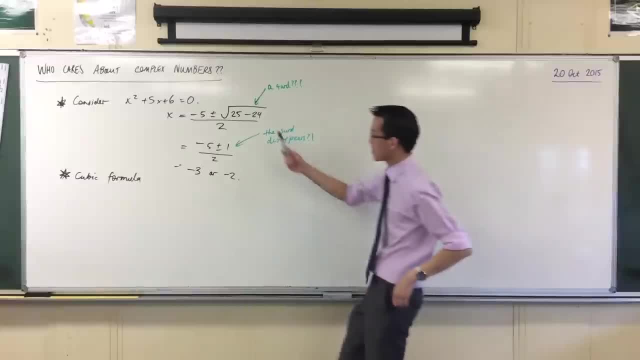 there is a cubic formula that exists, right, It's kind of you know. it's analogous to this kind of thing, except it's vastly worse. It's much longer. It like takes a whole page to write the whole thing across. 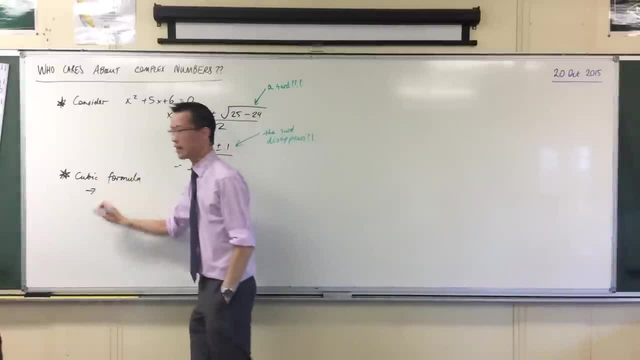 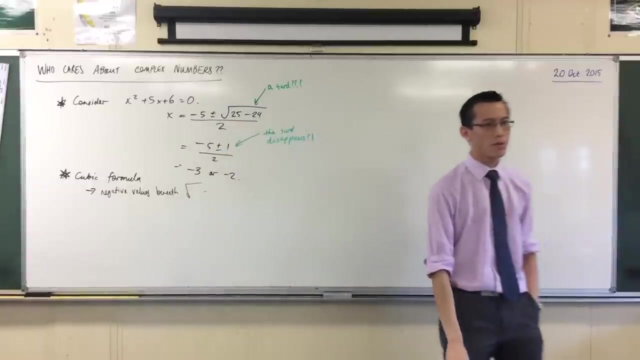 But more importantly, the cubic formula it includes. it's got baked into it negative values. underneath right, the square root signs that appear in it. right There are square root symbols, expressions in the cubic formula just like they are. 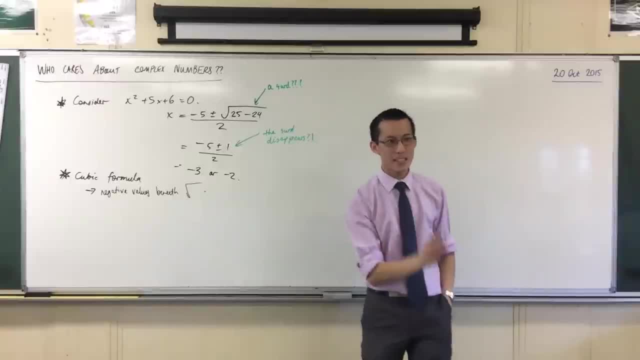 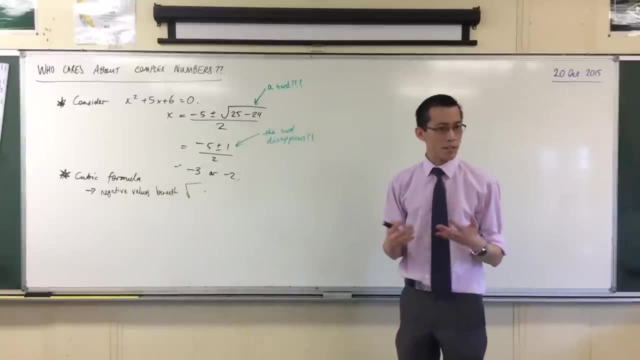 in the quadratic formula, but by necessity, the cubic formula has negative values under there. They have to be negative, okay. Now this is weird, though, because if I give you a cubic right, let's just consider a cubic like, say, I don't know. 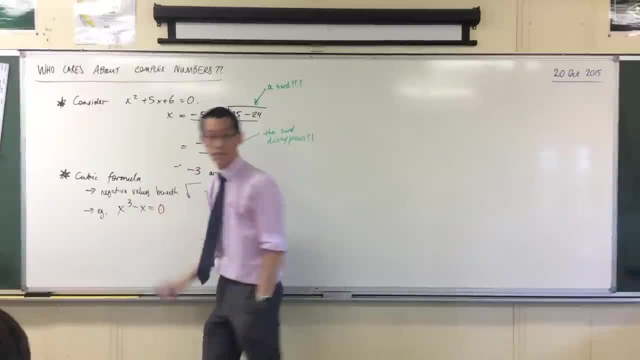 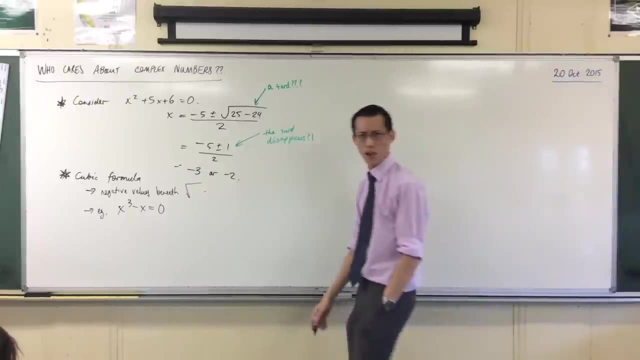 y, I'll just give it to you like this. Here's a cubic. I'll just give it to you like this: Okay, Now this cubic has completely real roots, right? What are the roots of this thing? Can you help me work them out? 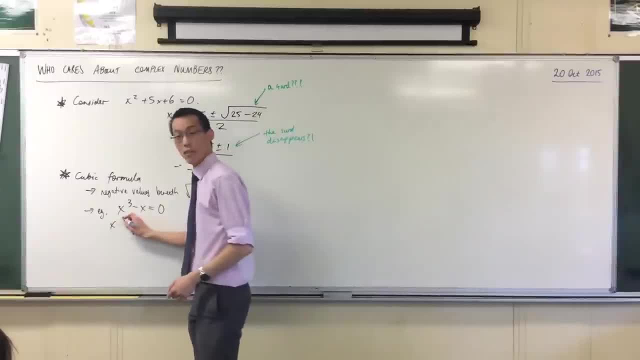 How would I work them out? I can factorize right, which gives me this Yes, And then I can factorize one more time, Do you agree with that? Which gives me x minus 1, x plus 1.. So this is a cubic. 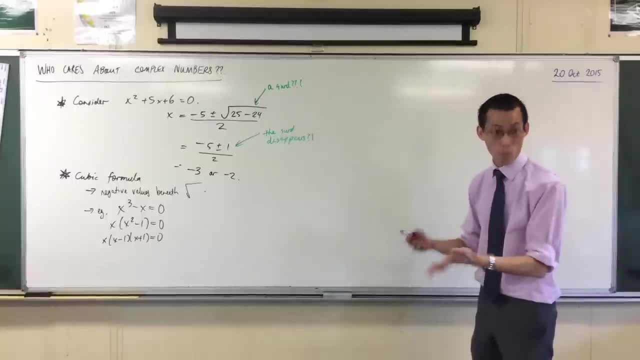 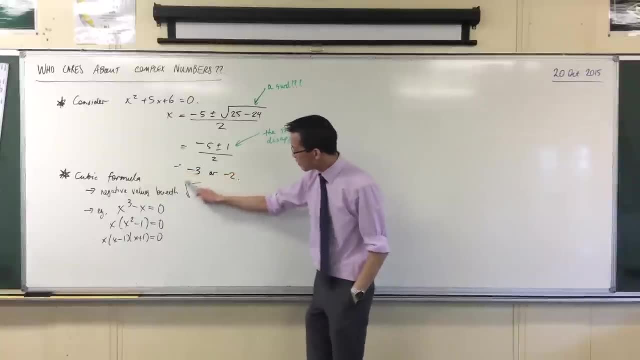 You expect it to have three roots and there they are, and they're all real roots. but in order to get to these real roots, you have to find the real roots. If you want to use the formula, negative values- non-real numbers- appear in the formula. 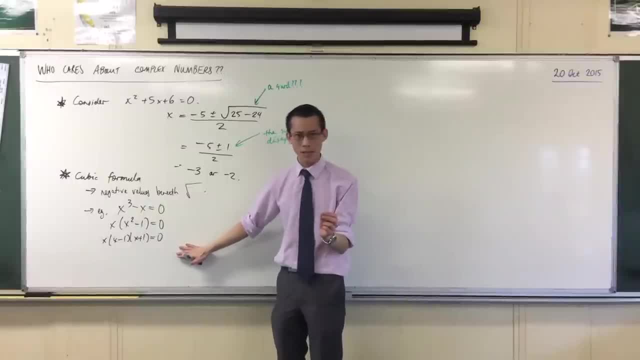 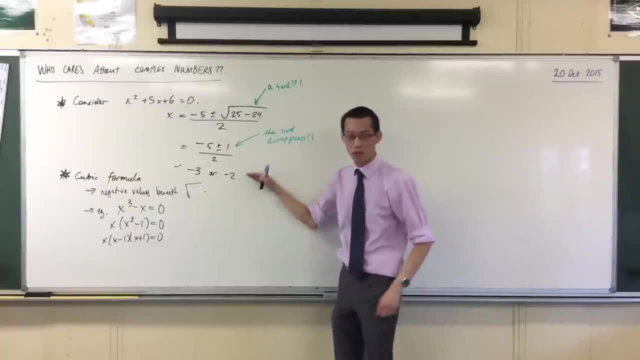 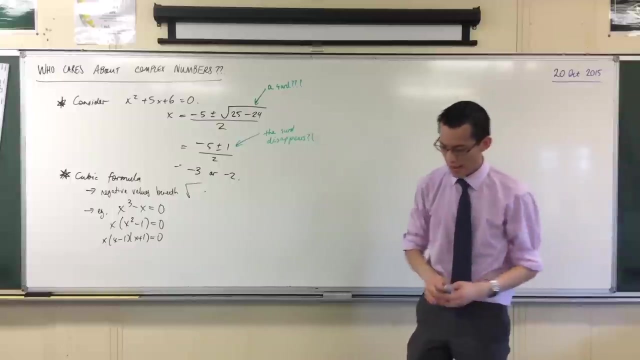 even though what you end with is completely real. Does that make sense? In the same way that irrational numbers appear in here, even if what you get at the other end is completely rational. Okay, Now, this is a very strange idea, and it gets at why numbers have the names that they do. 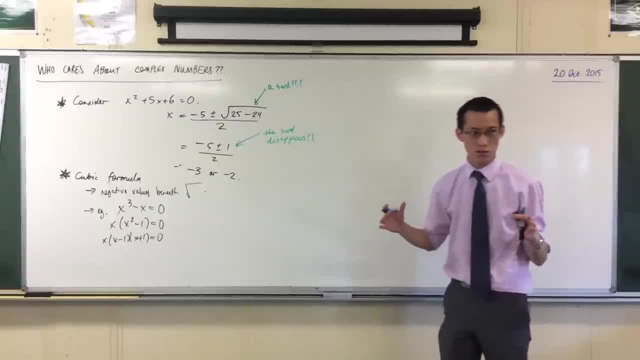 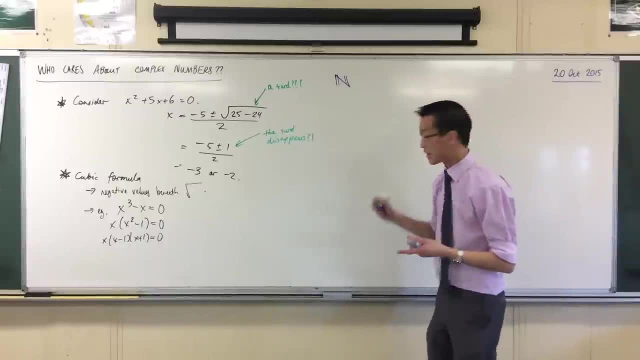 I want you to recall What were the families of numbers that I introduced to you before. Do you remember what they're called? We'll start with the natural numbers, right? And what was next after that? We talked about the integers, so we include negatives, right? 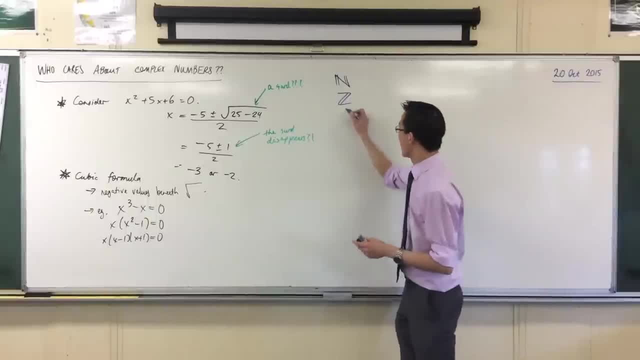 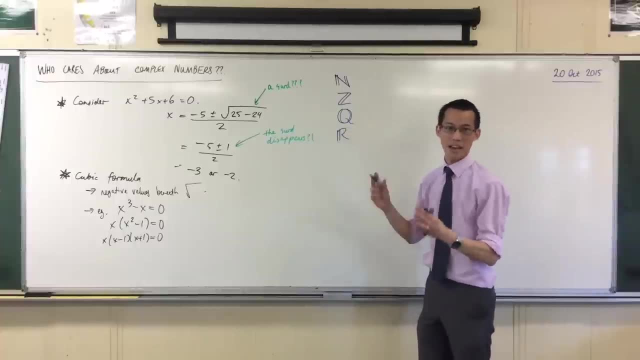 What happened after that? The cube one. We talked about rational numbers, right. Then we went to real numbers and then we've landed where we are, which is the complex world. okay, Now the important thing I want you to notice, right? 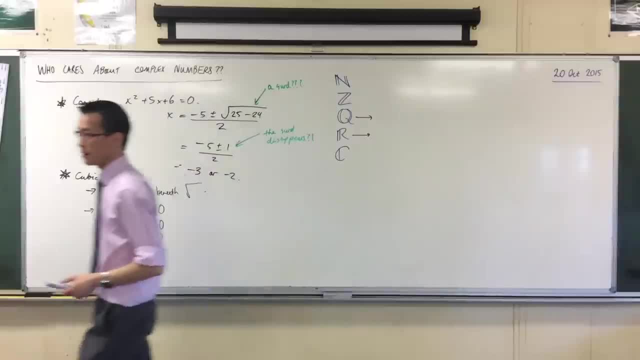 is that we've moved to the complex world. The point is that we know what rational numbers are and we know what real numbers are, but outside of these right, we have numbers in here that seem to be not rational and seem to be not real, and they've got these strange names. 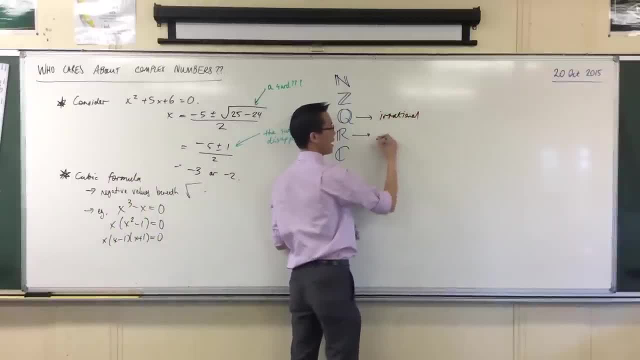 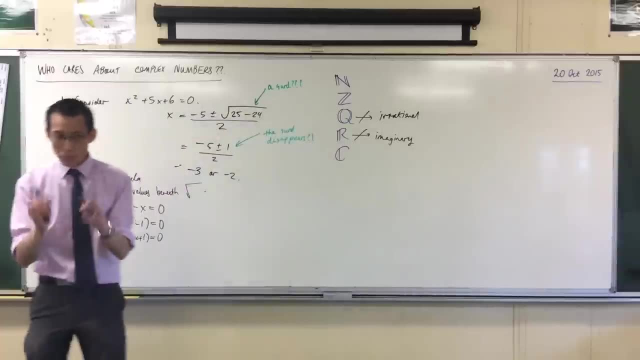 We call these irrational numbers and imaginary numbers. okay, if they are not in those sets, okay, Now just ponder this for a second right. If you were not in those sets. okay, if you were not a math student and you saw the word irrational. 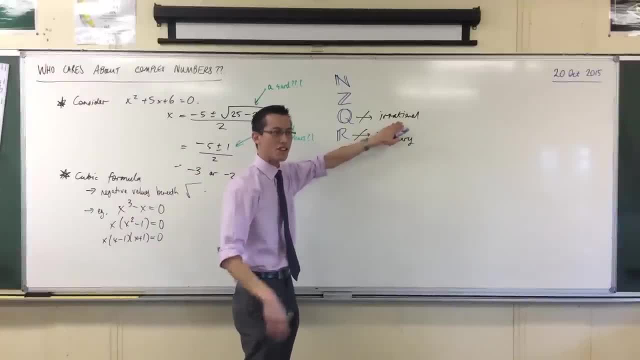 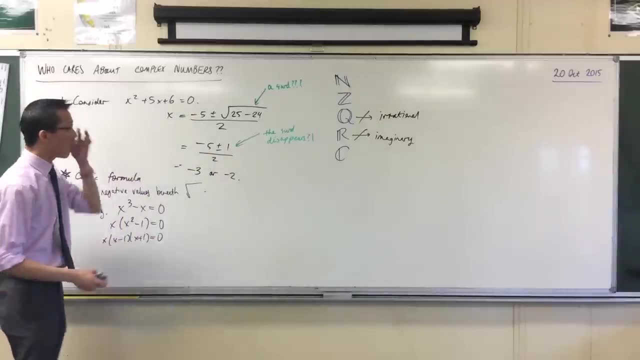 what would that mean to you? It would mean like: stop being irrational. It means stop being crazy, Stop like not making sense, right? That's what rationality or irrationality is, And the whole point is that the reason why that word means that is because in here, 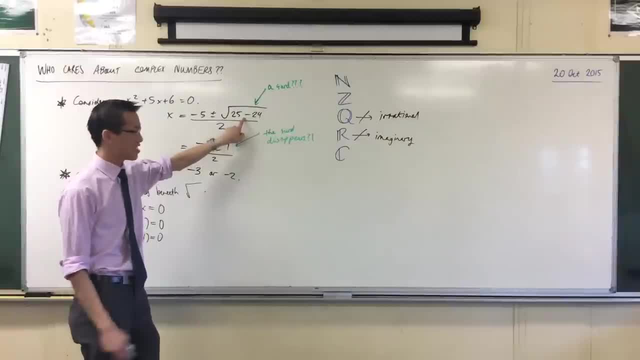 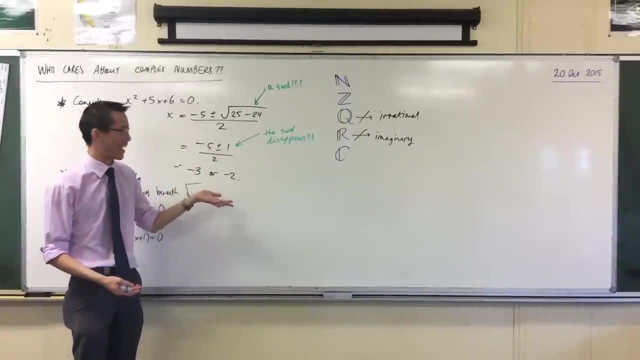 it's like you know what. this number doesn't really make sense. It's just stupid. It just disappears anyway, but we kind of have to put it in kind of as a hack, right? It just makes the formula work, okay. 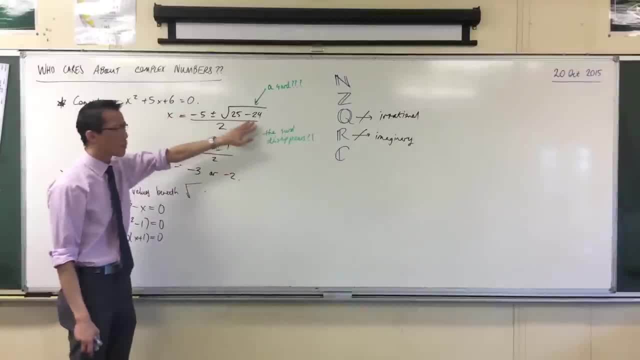 It's not real. If it's not really there, it'll disappear, but you've got to put it in at some point, okay, By the way, just as a side note, I brought this along with me because it's a really cool example. 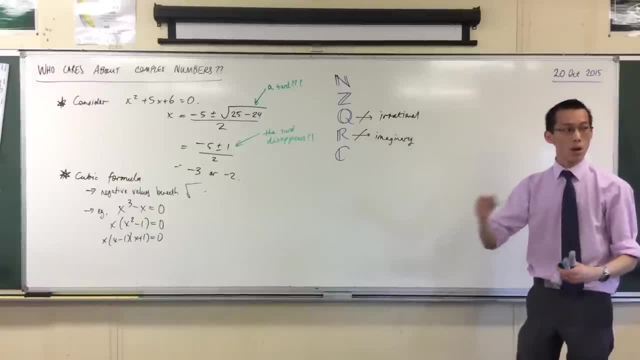 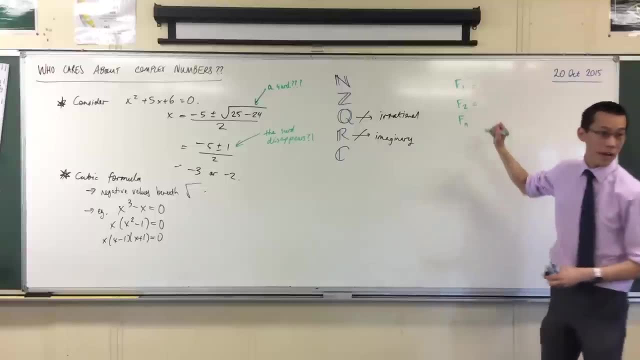 You guys know the Fibonacci numbers, right, The Fibonacci sequence. We have a definition, a recursive definition for it, right, It means F1 and F2, and then we can say: FN, Can you help me out, What's F1?? 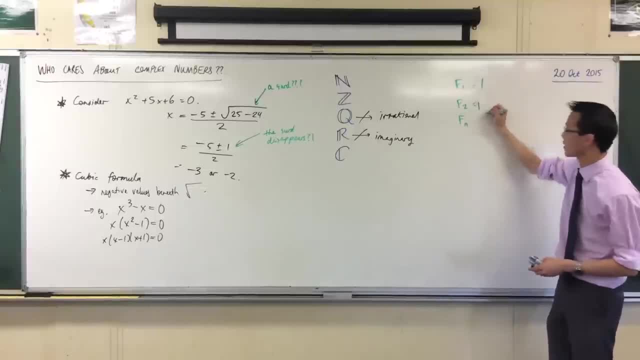 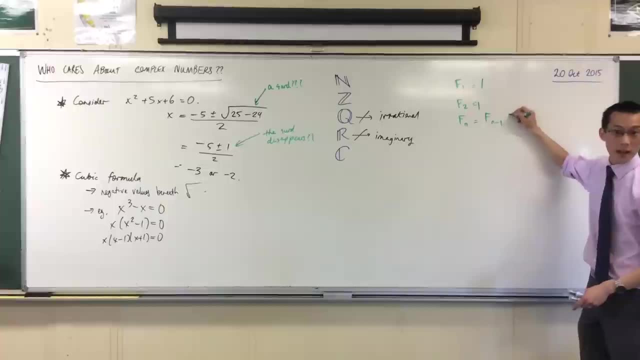 One, One, One. that's the first term. F2? Also one. Okay, once you know that you can write FN, What's the Fibonacci number? It's the previous one plus the one before that. okay, Now we've been working with series and sequences long enough to know. 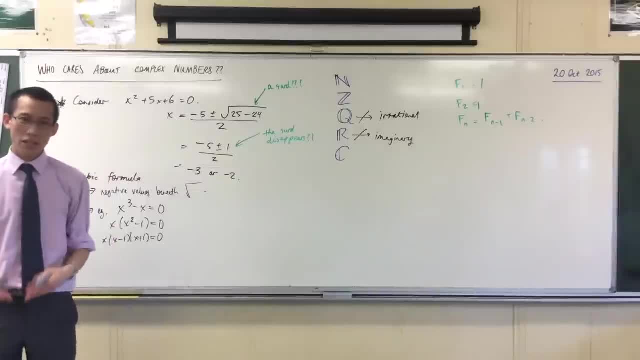 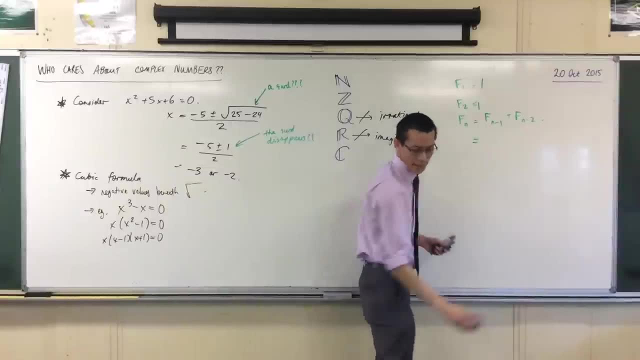 if there's a recursive definition, there should be, just like, a formula definition as well. right, We don't need to worry about it because it's outside the scope of the course, but it exists. It's this disastrousness. Is it plus or minus? 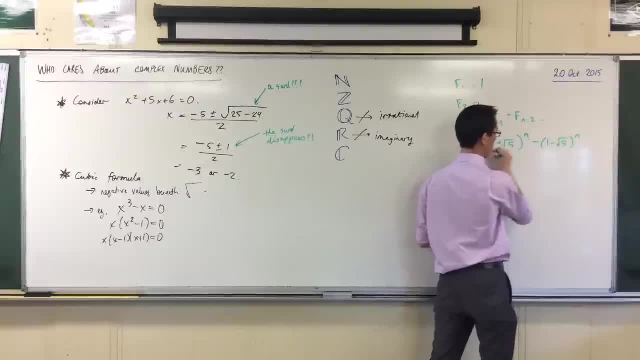 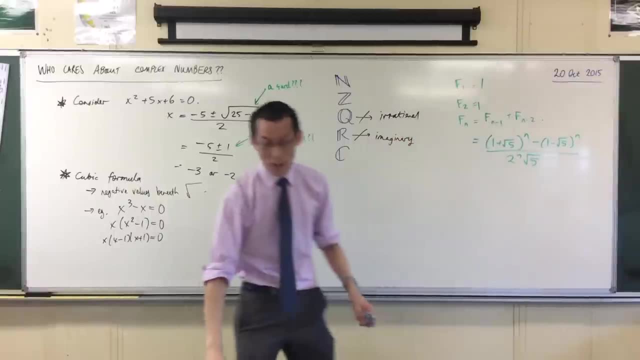 It's minus. Why is it? specifically Because it's root 5.. Good question, Because someone's The question for why it's root 5 has something to do with something important called the Gordon Ratio, but I'm not going to dig into it, okay. 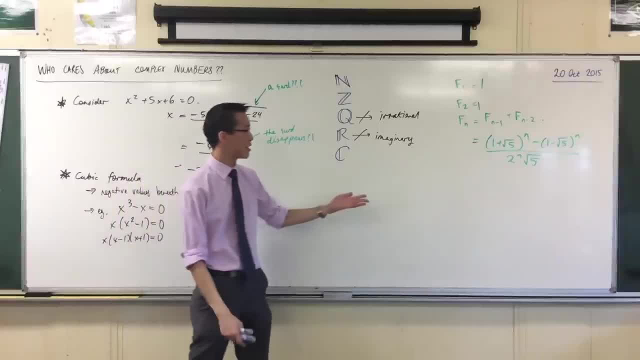 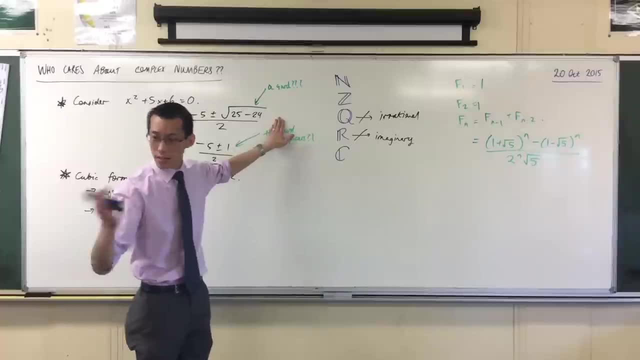 Now here's the really really weird thing. As you can see, just like with the quadratic formula, you can kind of understand why surds are in the quadratic formula, because you know what We know some quadratics- they do have irrational roots. 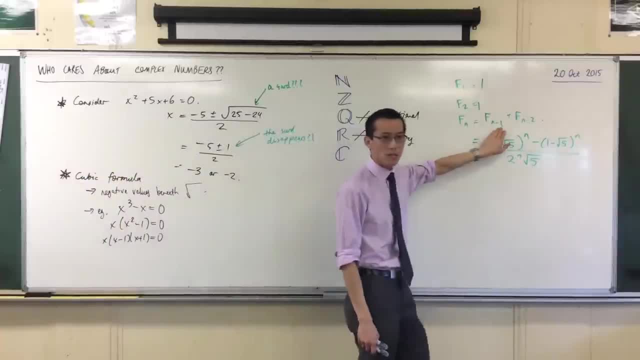 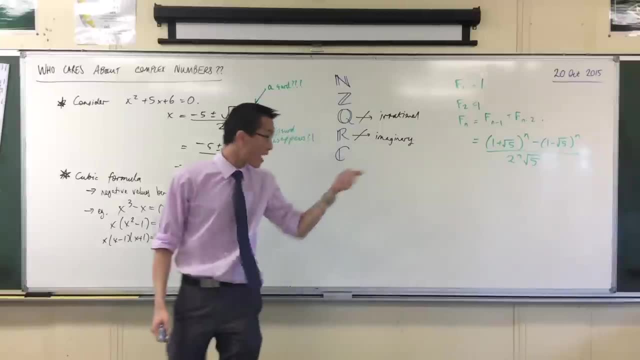 We know that. right, But there's not a single Fibonacci number. Okay, That has any irrational part to it. right, But you have to have irrational roots. You've got to have the square root of 5 in order to make the formula work. 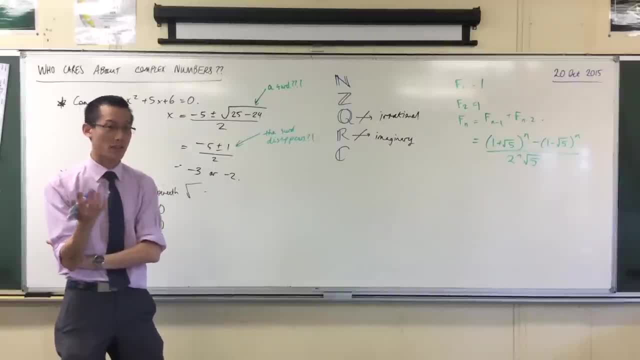 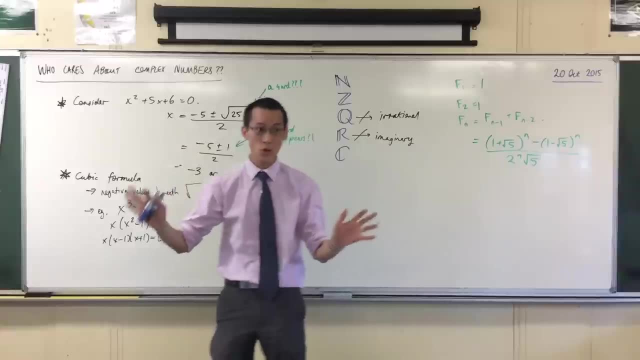 For any value of n. any, I should say any integer value of n, Actually any natural value of n. All of these squares of 5, they all come out in the wash, Every single one. They all disappear, And that's why you get this sequence right. 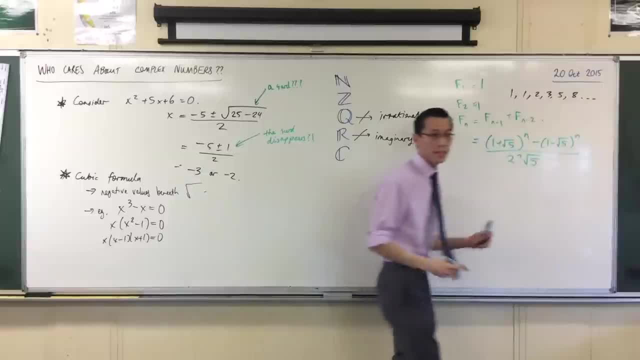 No square roots of anything to be seen. okay, But in order to make the formula work, you have to appeal to numbers that seem to be there like a hack, and then they disappear. okay, Now, that's why these numbers here, when you get negatives underneath. 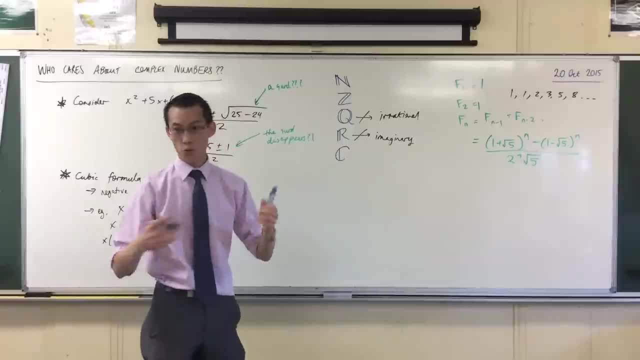 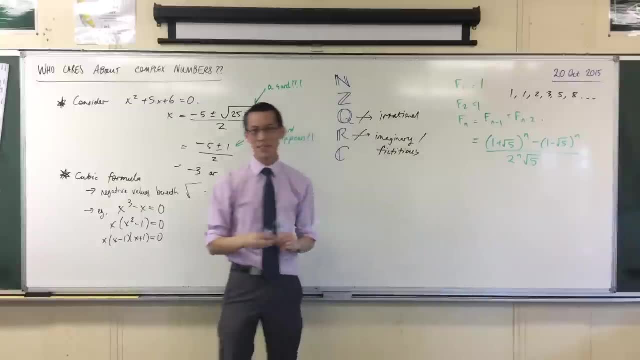 that's why they're called imaginary. In fact, the people who really pioneered in this field, they called them not imaginary numbers, but they called them fictitious numbers. They're numbers that they're not real. they're not actually there. 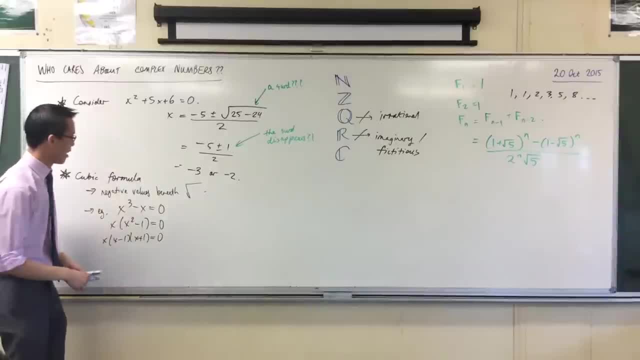 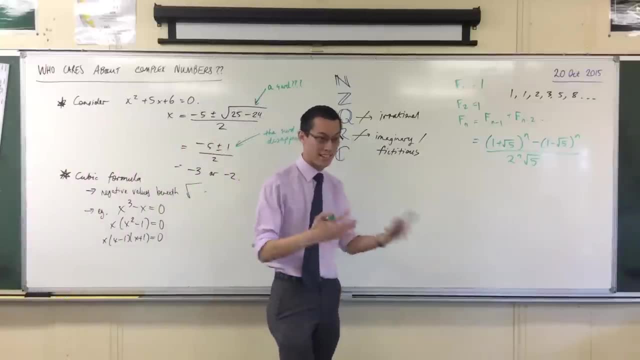 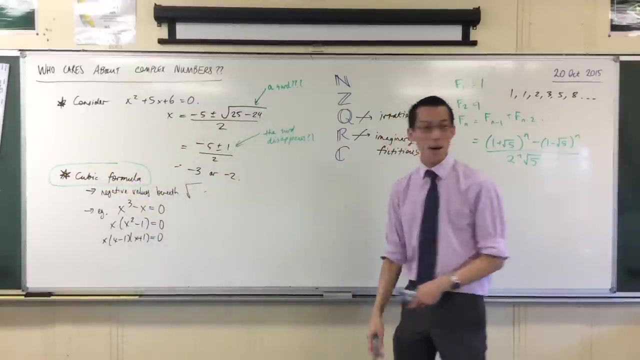 but you kind of need to stick them into your formula so your formula works. Question: Who is interested in such a thing? Who is interested in coming up with formulas that made numbers that didn't exist made them appear? And the answer is: and this is so interesting, you've got to go and look it up yourself. okay, 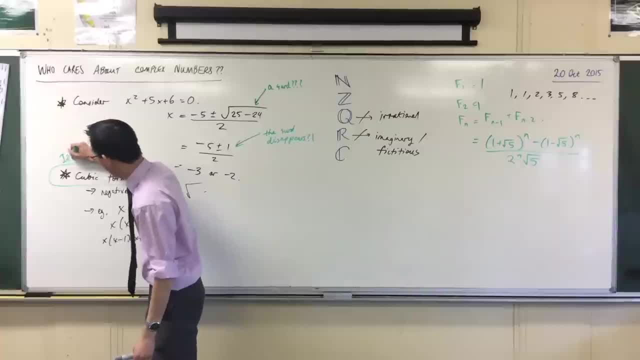 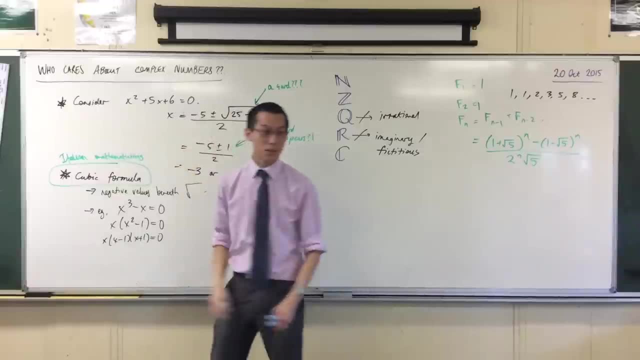 The short answer is: a whole bunch of Italian mathematicians. Now the one you want to particularly look for, if you want to go and search this up, because it's a hilarious story, as you'll discover in about 10 seconds. 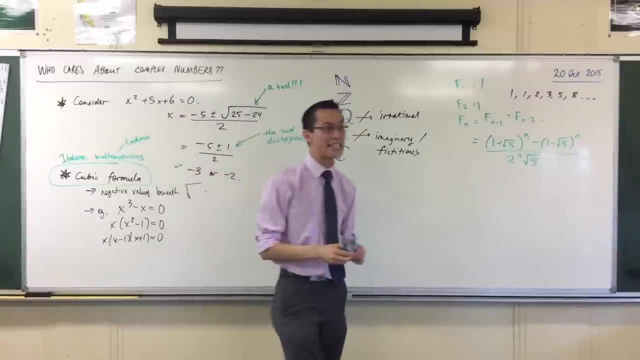 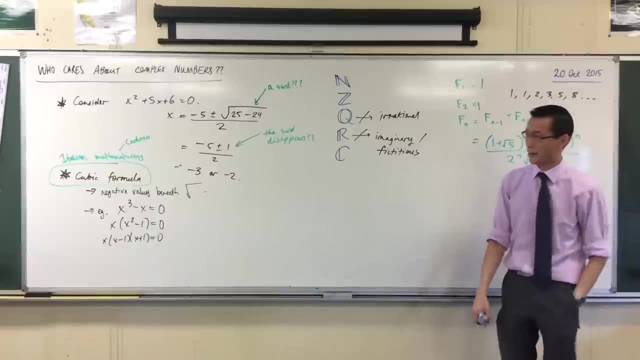 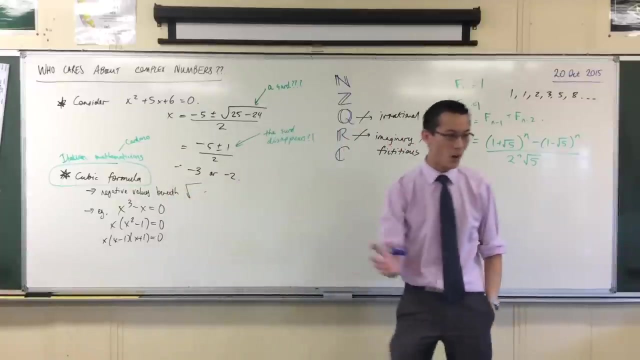 the one you want to look for is Cardano C-A-R-D-A-N-O, Very important Italian mathematician around the 1500s, 1600s, 1500s, 16th century, right Now. the reason this is such a big deal to them is that in the Italian mathematical world, 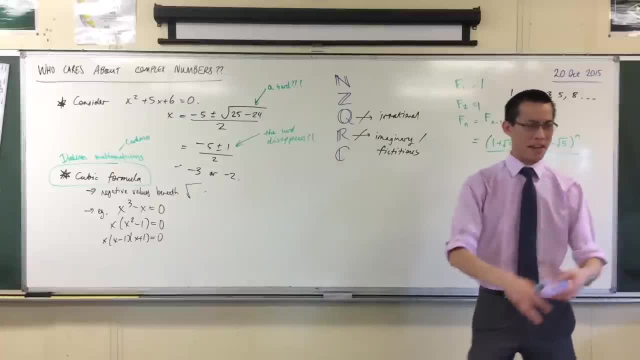 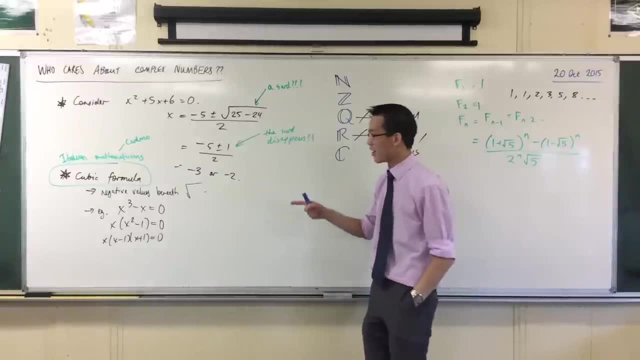 if you had like an office as the associate professor of mathematics or something like that. the way you applied for a job was you didn't put in a CV and then you had an interview process If you thought you were good enough as a mathematician to take that job. 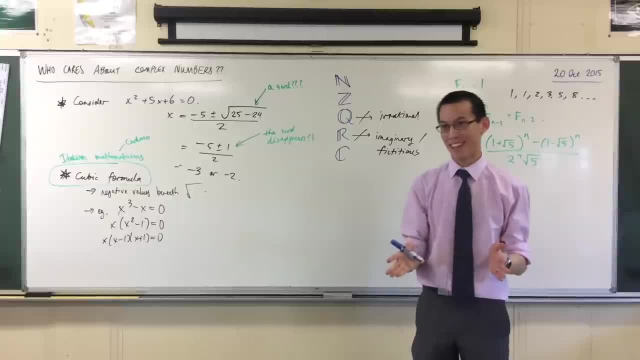 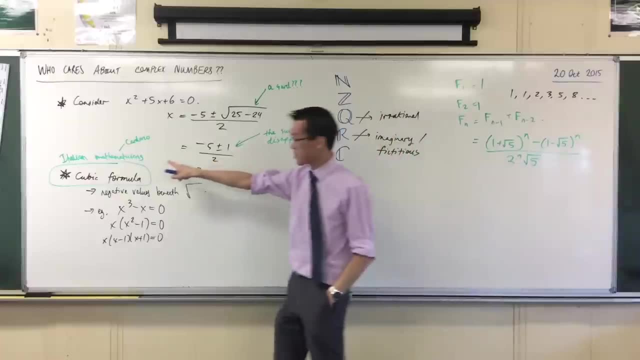 you challenged the person who had the job to a duel right Now, not just like any duel. Like the French people, they were all about bang-bang duels, right, But these Italian mathematicians? they had mathematical duels. 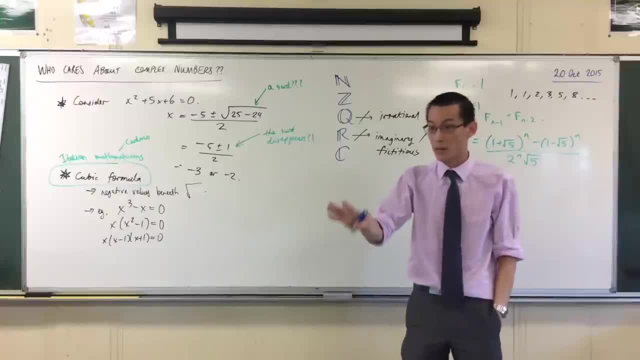 They were like: I think I'm a better mathematician than you and this is the way they would do it. They'd be like: look, I'm going to come up with 10 questions, right, and I can answer them. 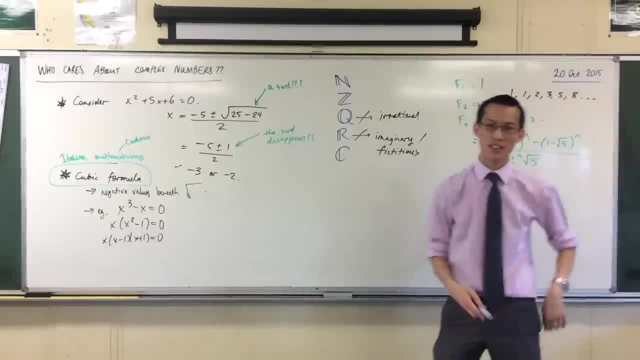 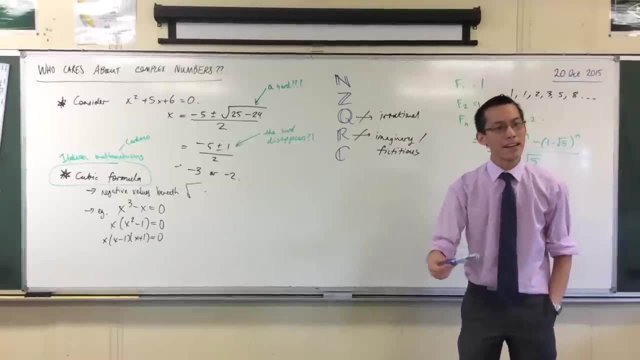 I know the answers to them, I'll give them to you. You give me your 10 questions. I reckon I can answer your questions faster and better than you can answer mine. What if they're like impossible? Well, as in the point is, I will give you questions that I know can be solved. 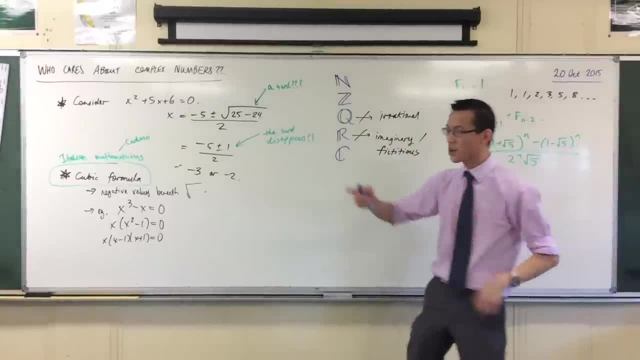 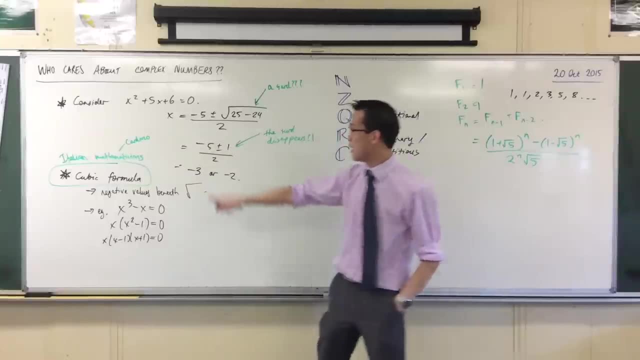 because I know their solutions right. So you can see, in order to win such a duel, there's literally like this mathematical arms race right Now. lots of people believed for a long time that quadratics could be solved, but cubics could not. right. 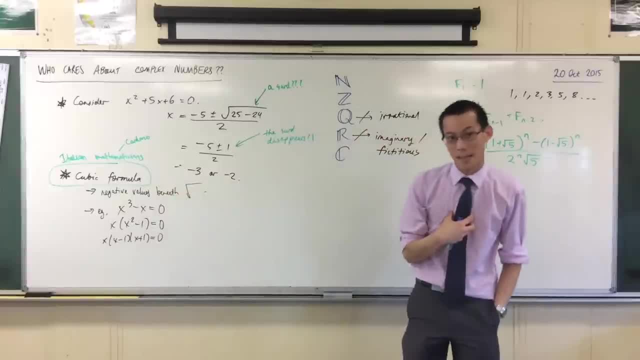 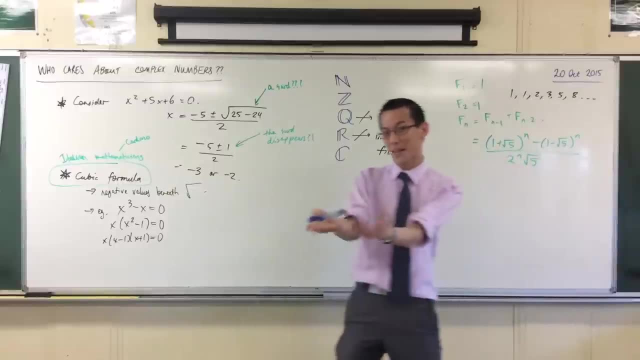 So it was like this holy grail of like: if I'm an Italian mathematician, right, and I can come up with a cubic formula, it's like the secret weapon that can shoot down anyone, because I'll give you a cubic and you won't be able to solve it, but I can right. 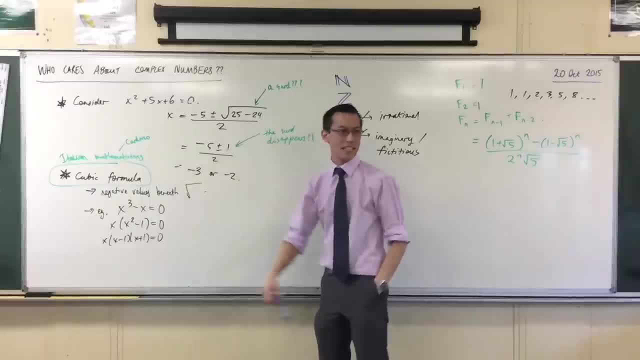 So they were intensely interested. They were interested in coming up with different kinds of cubics that can be solved. You know, for instance, monic quadratics are easy to solve, Non-monic ones are harder to solve, And it's exactly the same with cubics, right? 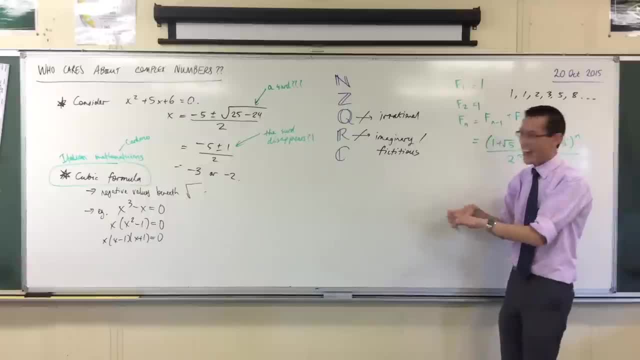 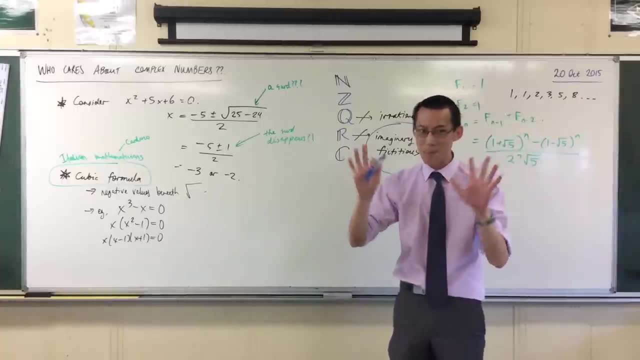 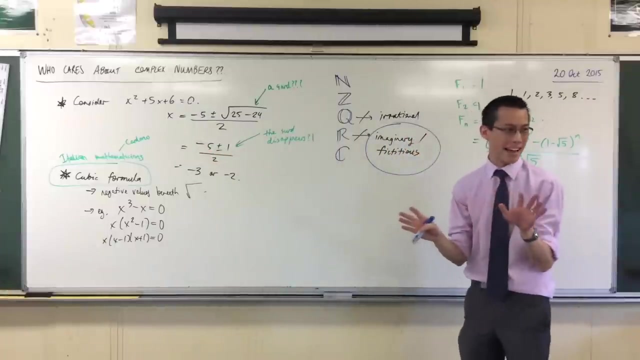 So that's why they pushed really hard into this area and they forced themselves to deal with these numbers, because that's how they could get someone else's job right And there were very, very prestigious positions. So you should look up Cardano and his duels and all the people he fought with and the secrets that were around. 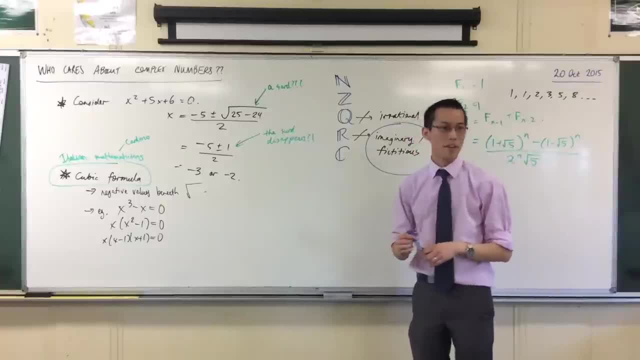 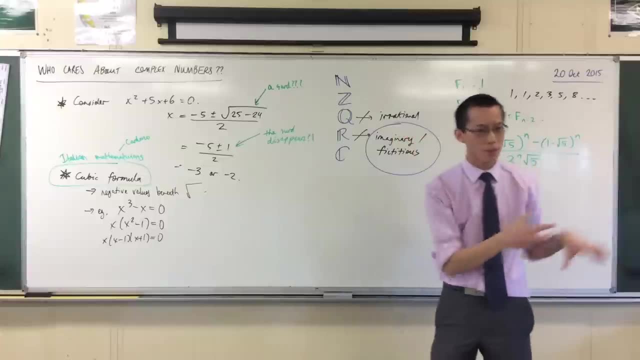 Did he figure out the cubic formula? He was one of them who did One of the tricky things. what's really hilarious is that you know how we talk about Pythagoras' theorem, and like theorems that are named after people, right. 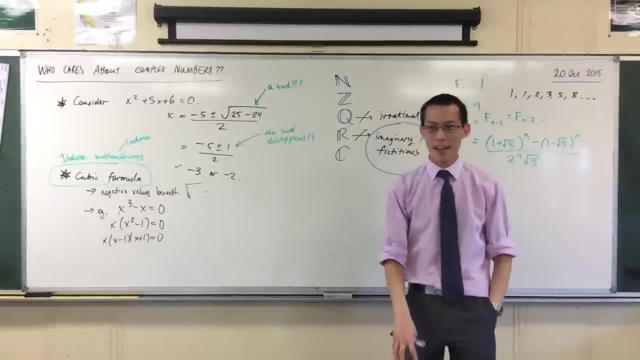 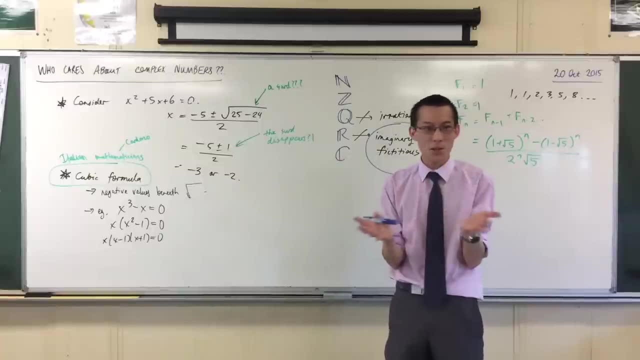 One of the reasons why a lot of the results that we have aren't named after people is because we don't know who came up with them. because they found a result and, instead of publishing it, they kept it secret, because that's your secret weapon. 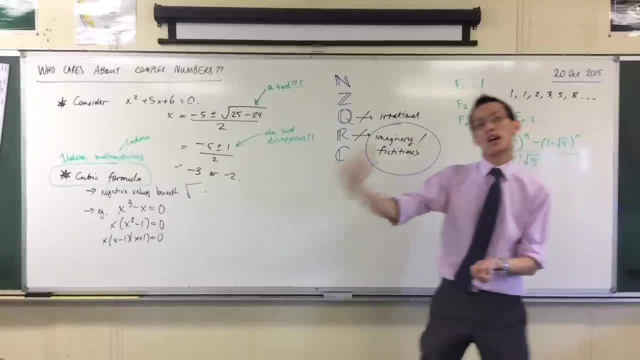 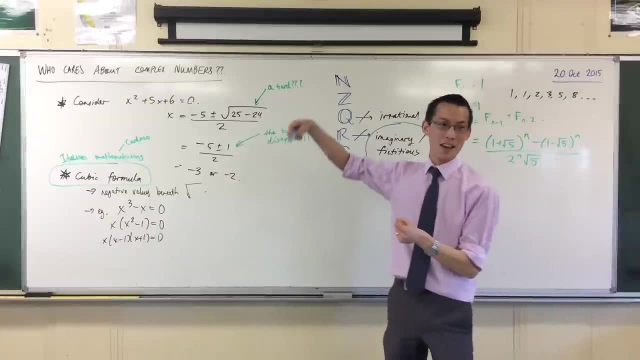 Why would you publish it, right? Yeah, exactly, So people would discover it, They would use it, They would win all these duels and then, when they died, they would take their secret with them to the grave. And then someone else, decades later, would rediscover it and be like: oh, this is cool. 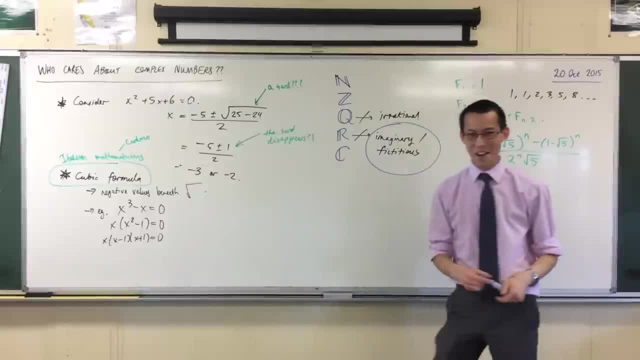 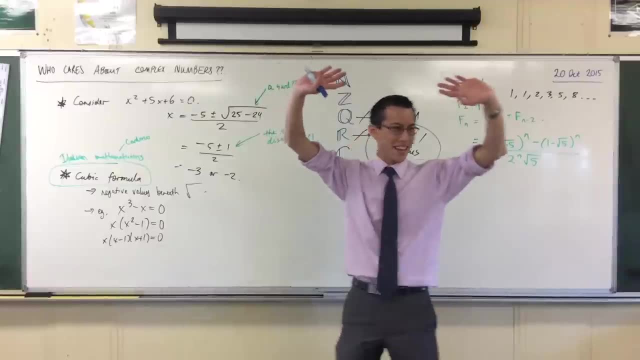 And then you know it was a lot of detective protection found out. That's really sad. So well, it just says something about the contract, Okay, so so, so, so, so right, Can we just come back? 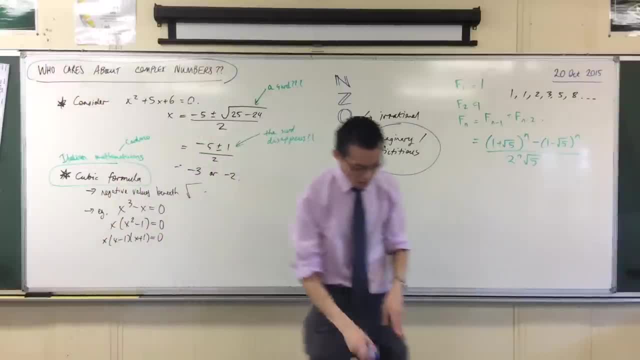 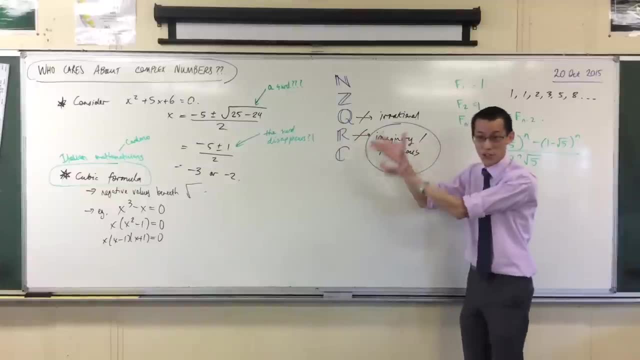 This is the question I was trying to answer, right. Why did people go to? Why did they want to go to, Like this field of numbers, which are so hard to work with? They are hard to work with, as you discover. 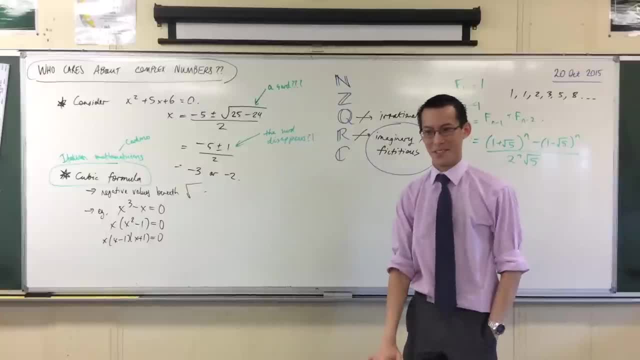 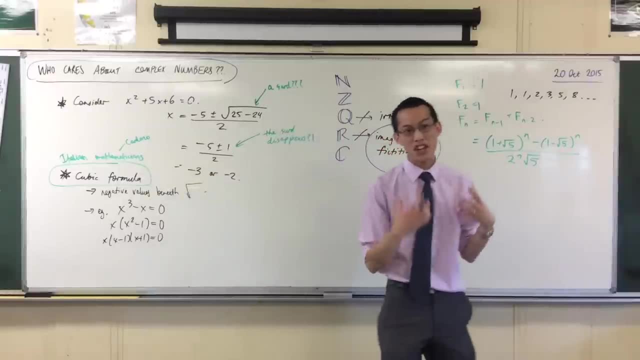 The answer is they didn't want to. They didn't want to go there, But in order to develop the weapons they needed, they were forced to go there. Because imaginary numbers. they arise naturally very quickly out of the regular old counting numbers.